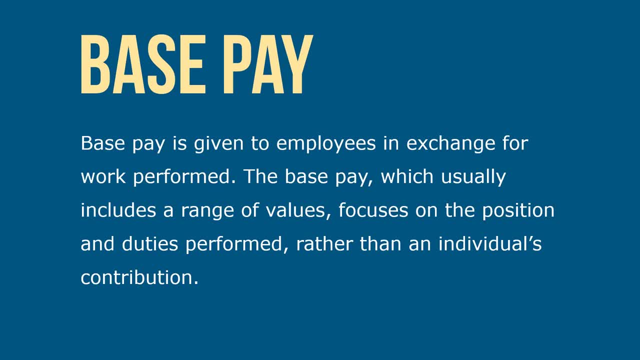 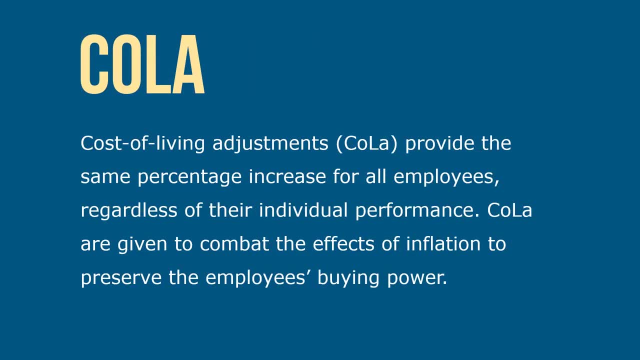 and duties performed, Rather than an individual's contribution. Base pay is usually the same for all employees performing similar duties. Cost of living or COLA adjustments provide some percentage increases for all employees, usually the same percentage amounts, regardless of their individual performance. 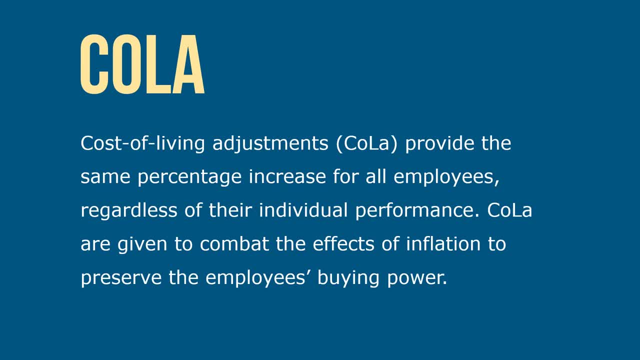 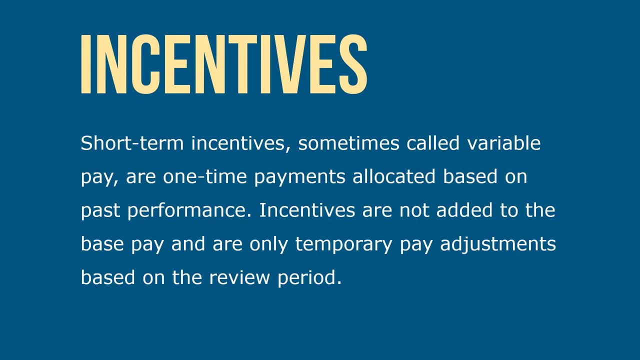 COLA are given to combat the effects of inflation and to preserve an employee's buying power. Short-term incentives, Sometimes called variable pay, are one-time payments allocated based on past performance. Incentives are not added to the base pay and are only temporary pay adjustments based on. 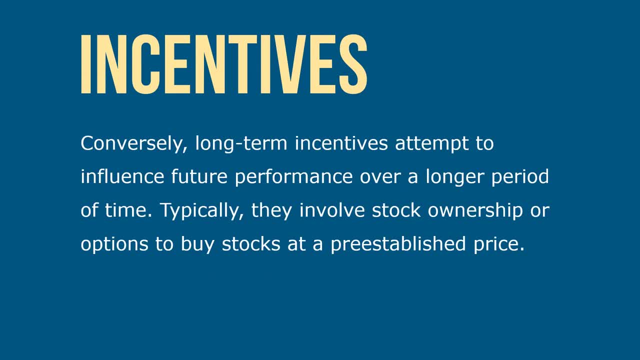 the review period. Conversely, long-term incentives attempt to influence future performance over a longer period of time. Typically, they involve stock ownership or options to buy stocks at a pre-established price. This investment is expected to translate into long-term payments. Incentives are not added to the base pay and are only temporary pay adjustments based. 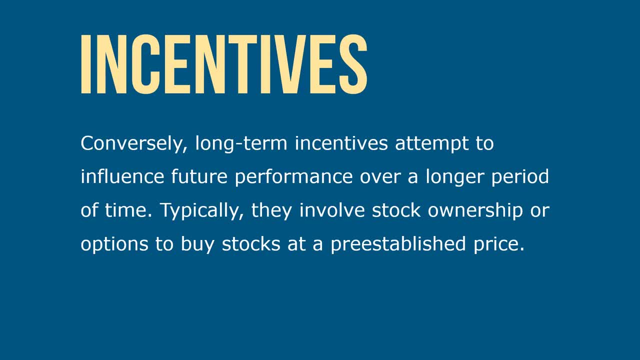 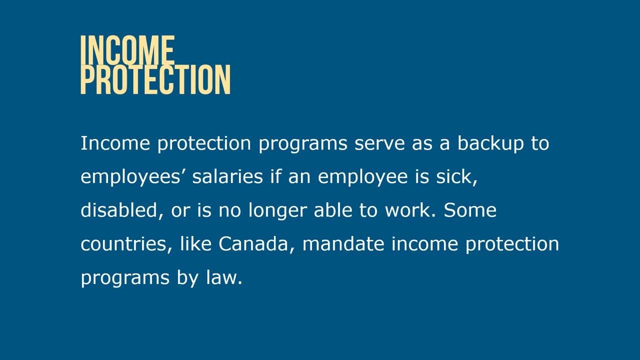 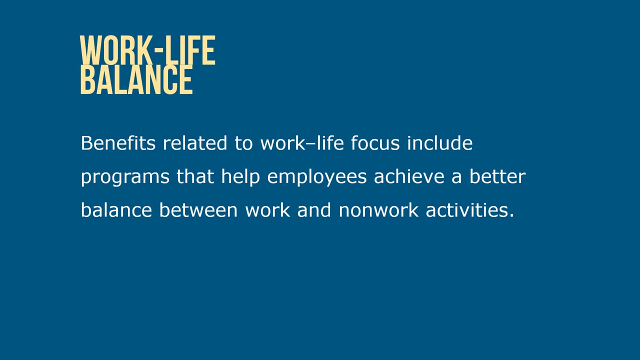 on past performance. Income protection programs serve as a backup to employees' salaries if they get sick, are disabled or are no longer able to work. Some countries, like Canada, mandate income protection programs by law. Benefits related to work-life: focus on programs that help employees achieve a better balance. 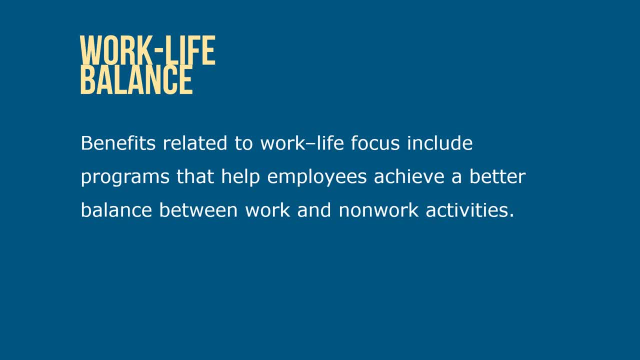 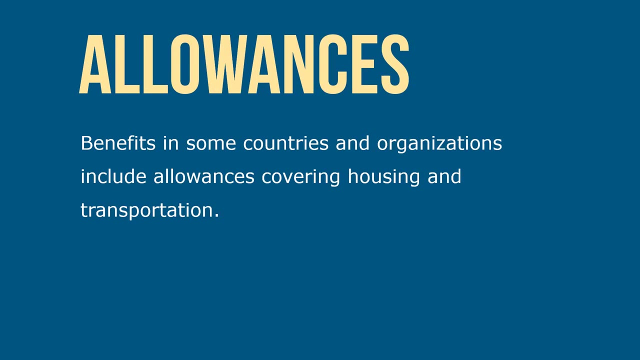 between work and non-work activities. These include time away from work, Like vacation time, Services to meet specific needs like counseling or financial planning, And flexible work schedules like telecommuting and non-paid time off. Benefits in some countries and organizations include allowances covering housing and transportation. 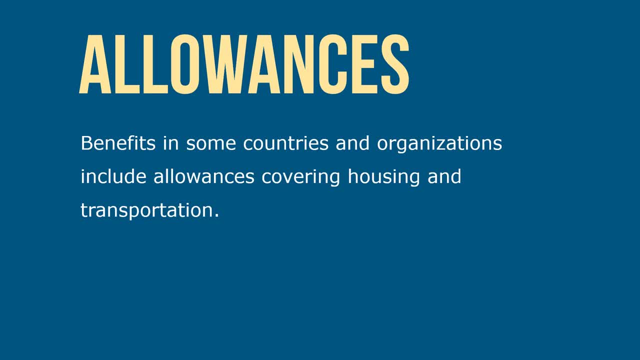 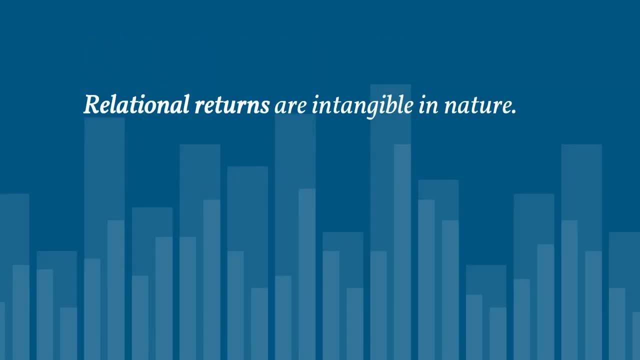 These kinds of allowances are typical for expatriate personnel and are also popular for high-level managers throughout the world. Relational returns are intangible in nature. They include recognition and status, employment security, challenging work, opportunities to learn and form personal relationships at work.